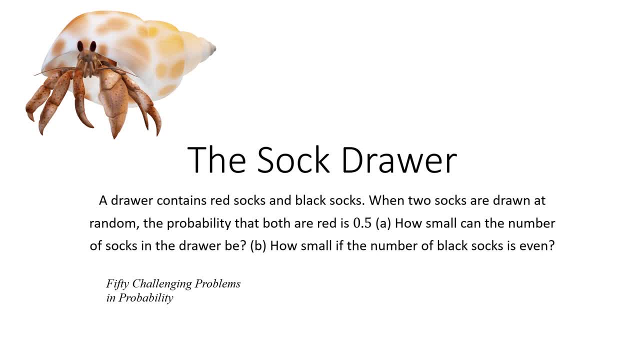 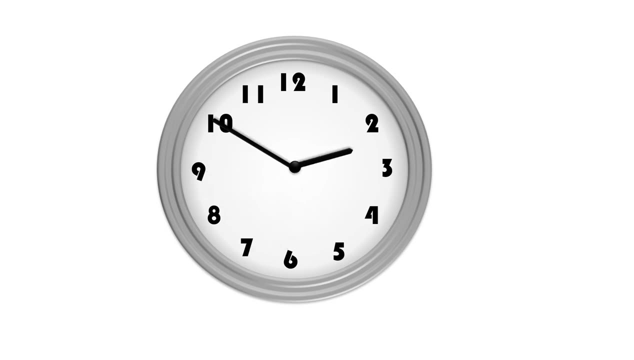 And I want to ask: how small can the number of socks in the drawer be? and how small if the number of black socks is even? Okay, so you can take your time and if you are ready, then you can watch the solutions. Okay, so this problem is very easy, So we can assume that there are. 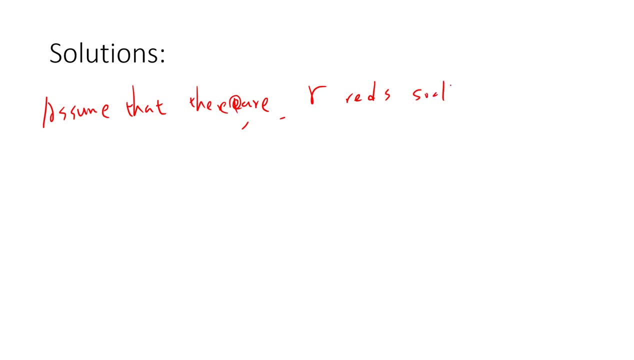 R red socks and B black socks in the drawer. So what we have is we take R- choose 2, and then we take the total R plus B choose 2.. This is the probability. what we take. Both are red. This is 0.5.. So we can write down the equation. 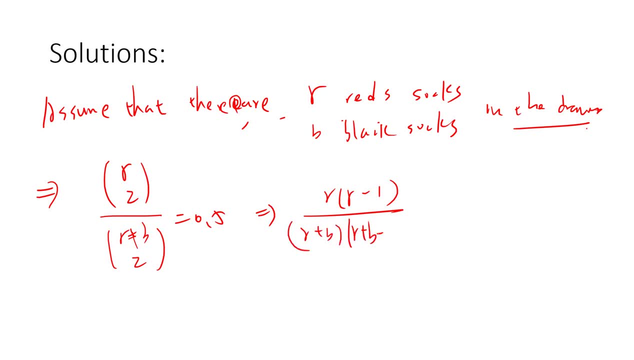 What I, what we have here. So we can write down the equation: What I, what we have here, We need to satisfy. So this satisfies 2 times R minus 1 minus R plus B, times R plus B minus 1 to be 0. 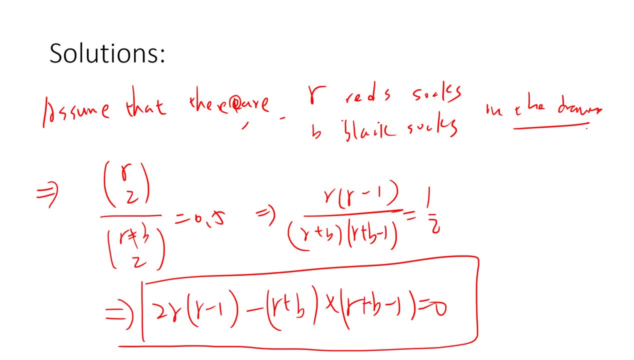 And then this equation is what we want to satisfy. What we want to satisfy, and both R and B should be positive integer or the natural number. Okay, so you have multiple ways to solve it. Basically, you can plug different R and try to solve for different B, or try to plug different B and try to solve. where you can get R is as an integer. 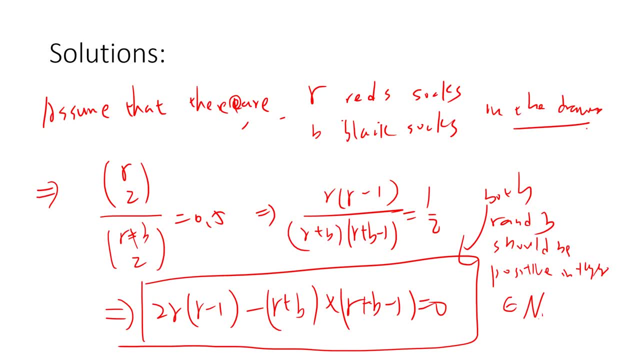 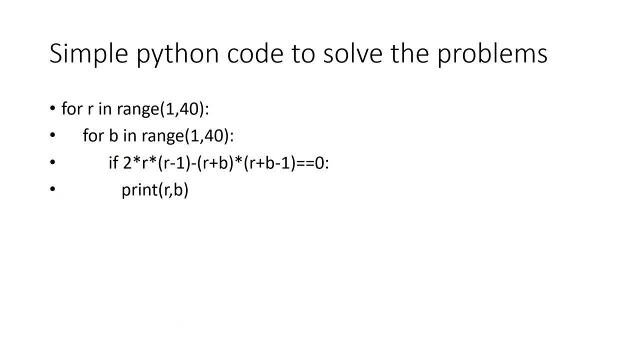 But the simple solution is to just write down a Python code and you can check. Okay, so what I write is a simple Python code. I just check for R to 1 to 40 and check B for 1 to 40 and I check out whether a low solution satisfy the Dolphin T equations or satisfy this integer. 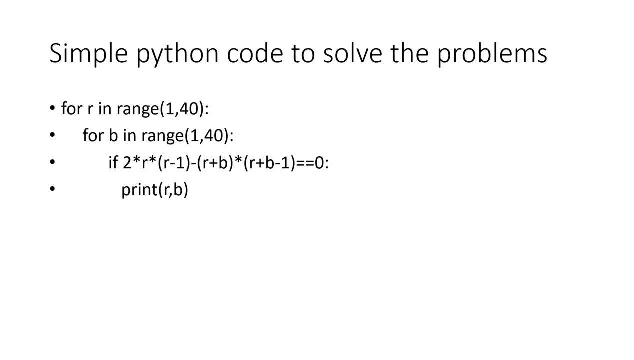 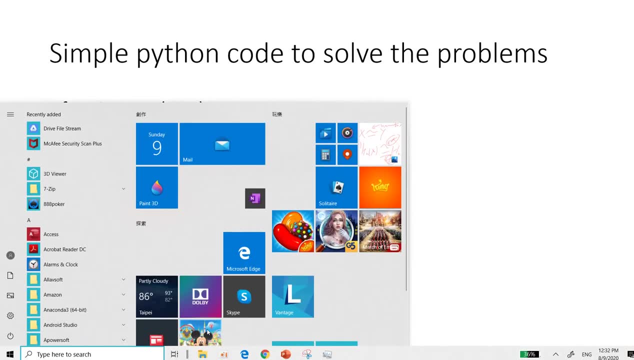 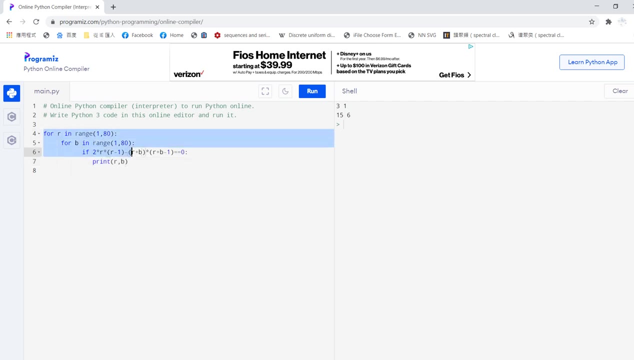 If this is correct, then I just printed a solution, So I just search for this particular range. Okay, so how about we go to see online Python code? So I know Python compiler. I just plug the answer. In this case, I solve 1 to 80..